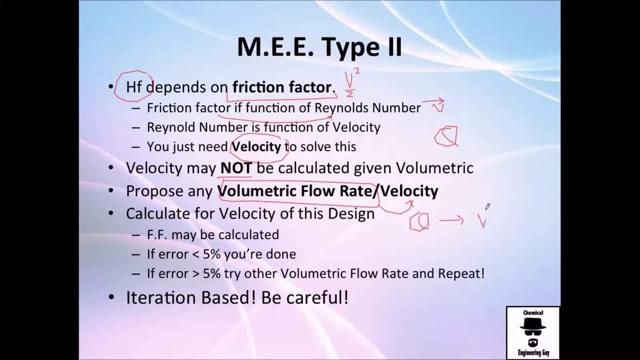 to give several volumetric flow rates and calculate velocities. With these velocities we're going to calculate left side of mechanical energy equation and calculate right side of the mechanical energy equation. If they make sense we're set to go. Just be sure to be very low in error. If you have a small error you're done. If you have a high error, 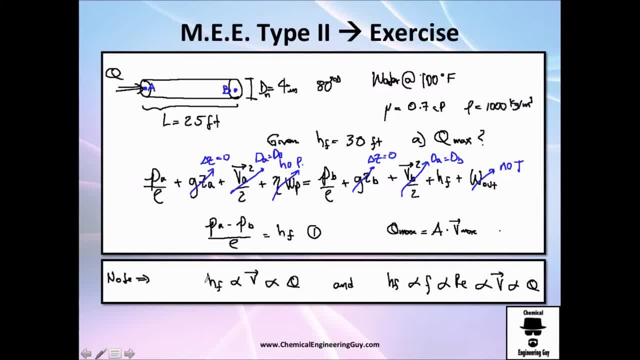 you must retry. So let me explain you this problem. I took one simple problem so you could get the idea of what is type 2 problem. I got a volumetric flow rate which I don't know in point A and point B, The length of. 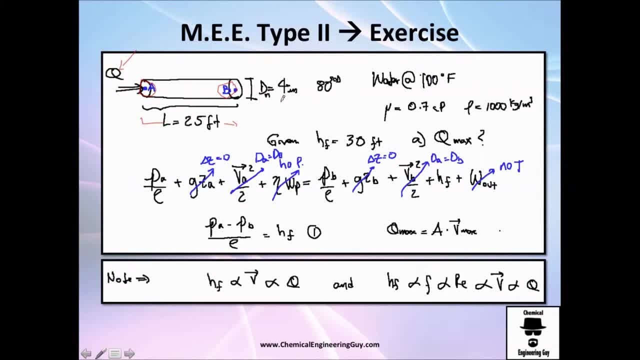 the pipe is 25 feet, The nominal diameter is 4 inch. in a Fourier schedule, pipe Water is at 100 Celsius Fahrenheit. So I calculate the viscosity and the density right here And they tell you that the maximum amount of, let's say, friction drop is this one. So 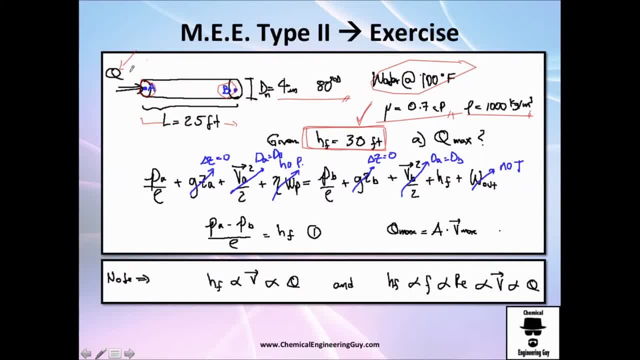 that's good Because we don't need to calculate. but we still need to calculate the volumetric flow rate. So they ask us if 30 feet is the maximum friction to let's say to have, we need to calculate the maximum flow rate. So let's do a balance: Since same height, I can cancel. 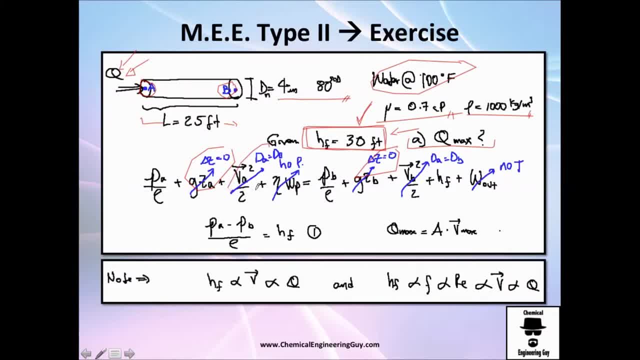 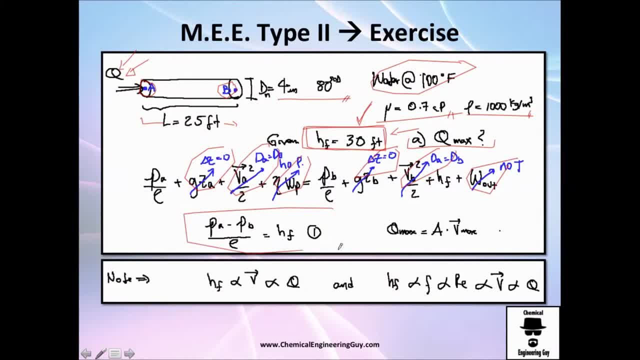 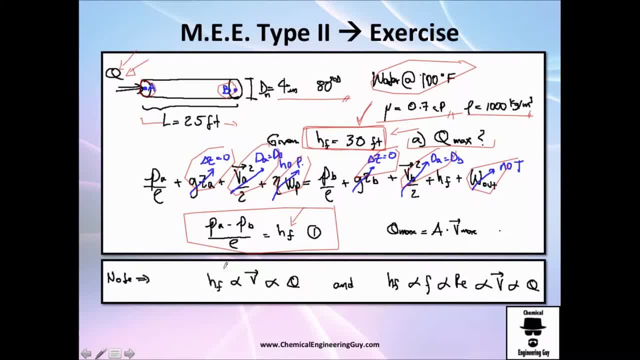 rate equals area times velocity, And please have a note that this depends on the velocity, which depends at the same time on this, And that the friction factor depends on friction and the friction F depends on Reynolds. Reynolds needs velocity And velocity comes from Q. 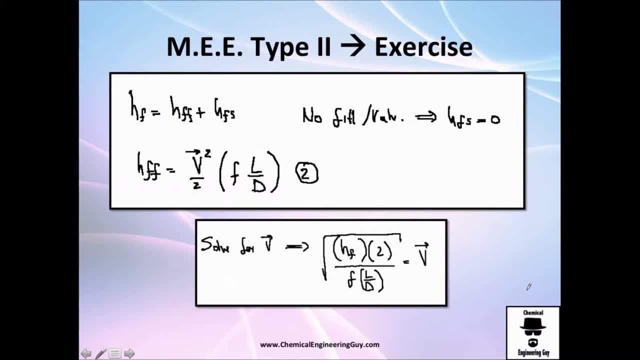 So, guys, if I need to do this, then I'll do an approach. Let me calculate the energy loss. So, doing this, do the wall. I have no fittings, Actually here, no fittings, no walls. HFS is equal to zero, so i get this. so one trick i can do is- since i know i want to add an extra equation- 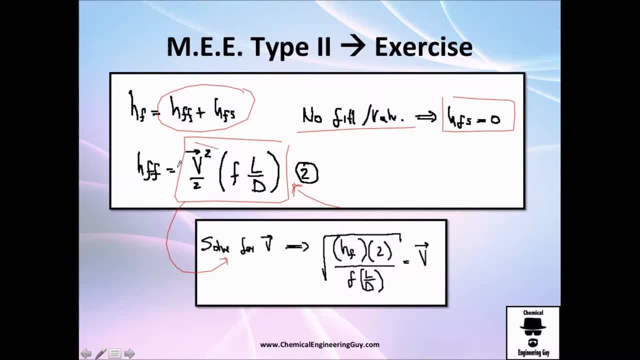 so i know, the wall, the wall loss is this one i can solve for velocity in this case. this one, i have it, this one, i do not have it. this one, i have it. no, i don't have this and i do have this. so let's go. 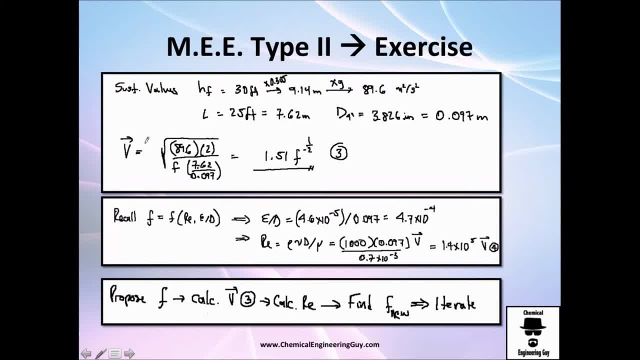 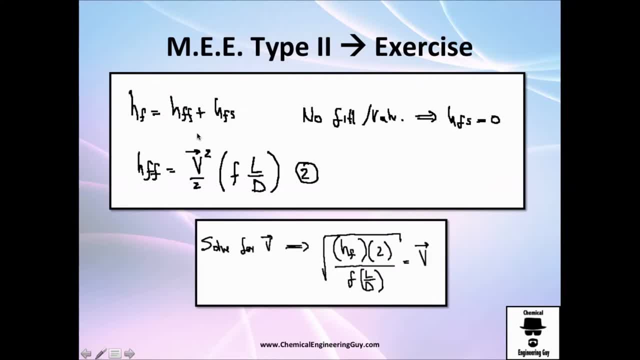 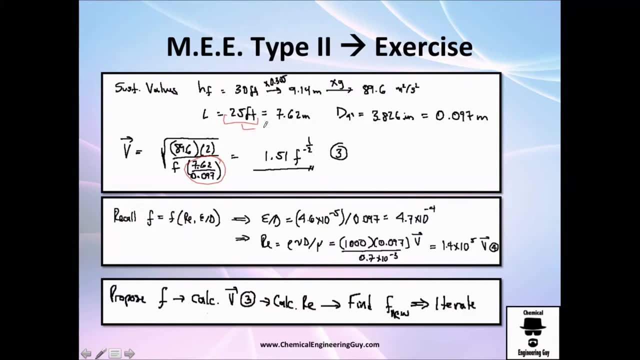 and you get that velocity equals to this value. if you substitute every data, you have hf here you have. well, this two is from. this two is constant. i got the length and divided by diameter, the length we call is 25 meters, not 25 feet, about 7.6 meters. and i got this equation, equation number. 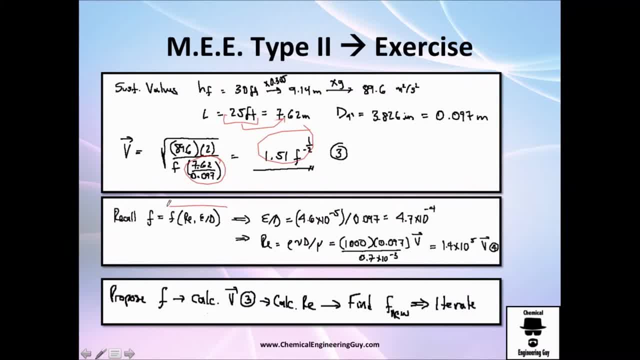 three, and i recall that the friction factor, or factor of friction, is function of Reynolds and relative roughness. so let me calculate that relative roughness is d roughness divided by the diameter, which i got to be this one right here, and the Reynolds number. i cannot find velocity, but i can substitute everything. 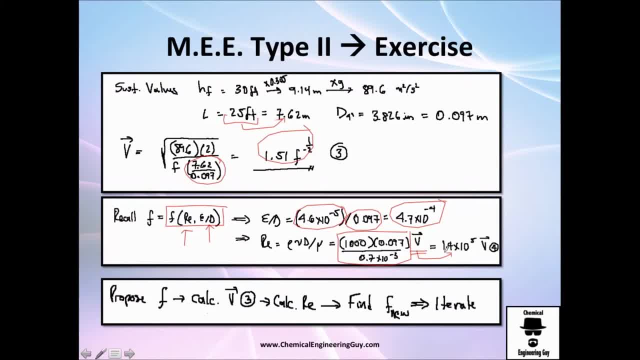 in function of velocity. so i get equation three and four. so let me explain you what is my idea. i'm going to propose an f value, then i'm going to calculate velocity from here. once i got velocity, i can calculate the Reynolds number from here. and once i got the Reynolds number, i can find the new friction factor in the Moody's diagram. 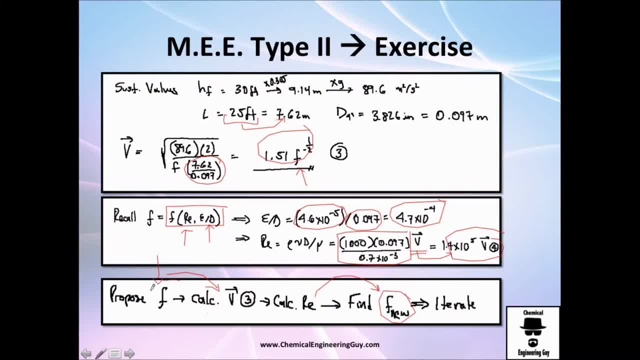 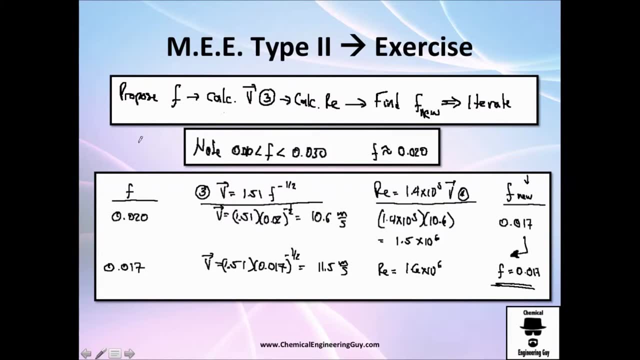 and if this friction factor is pretty near to the friction factor i guessed, then i'm done. if it's very far away, then i need to iterate, okay. so before i just doing random uh f values, recall that the typical application is between zero and 30, more near into or, more commonly, between these numbers. right here, 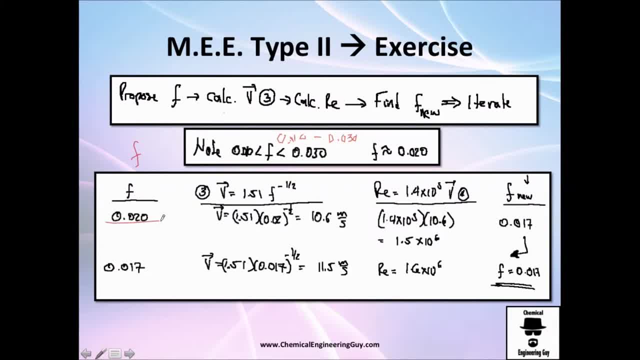 so let me choose 20 as a base. so i propose a friction factor. i substitute in the equation of velocity, right here i got a velocity which is, i think, very high, and then let me calculate the Reynolds number with that velocity. i got 1.5. and since i already got the relative roughness right here, 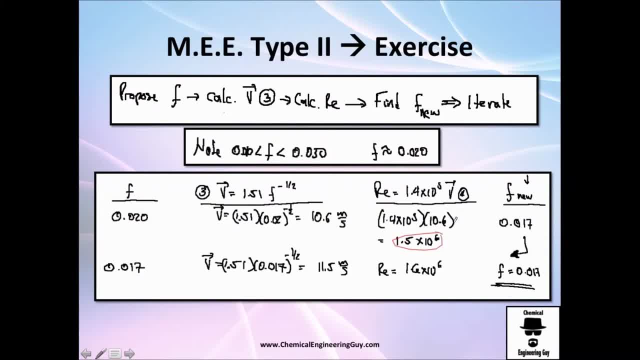 and i got the Reynolds number. i find out that my new value of f equals 0.17, so it's a little bit less. i will use this value right here and do the thing the process again: calculate velocity from the value 17, i got 11.5 meters per second. calculate Reynolds number is almost the same. and now i check. 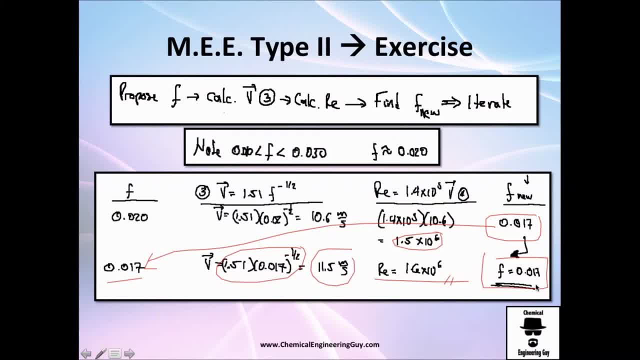 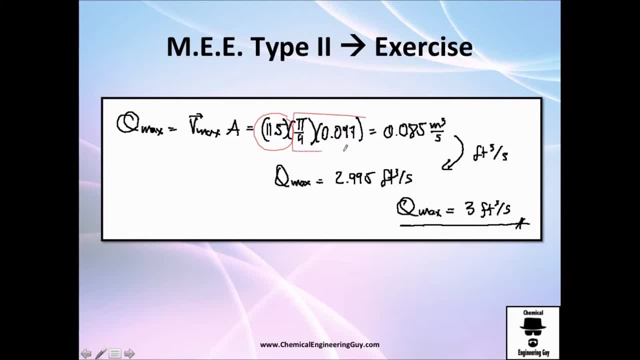 out and my friction factor is the same. so i can say this is my final answer, since velocity, i guess, is 11.5. now i can calculate the, the volumetric flow rate, because i already know the velocity and the area. i got this one: 0.085 cubic meters per second. 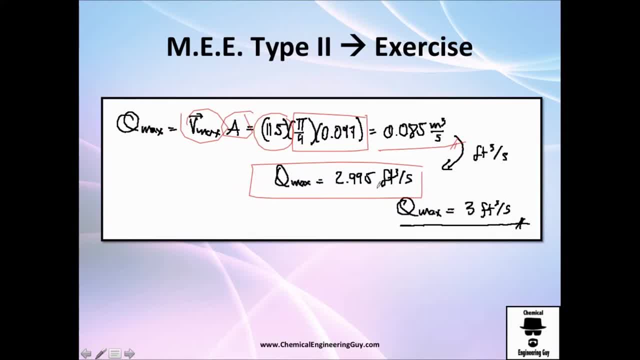 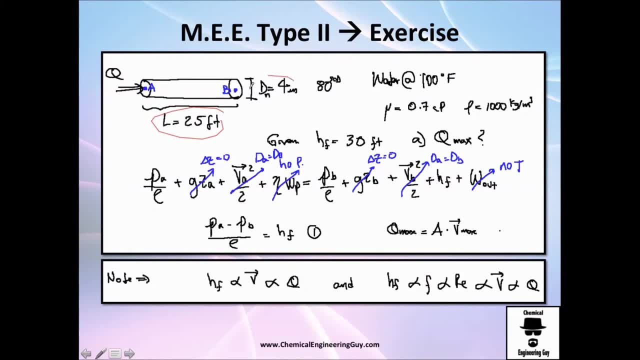 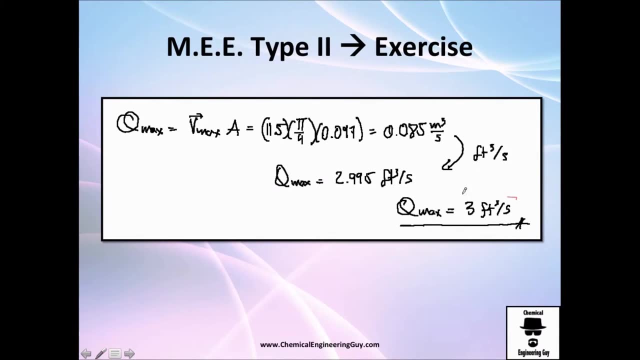 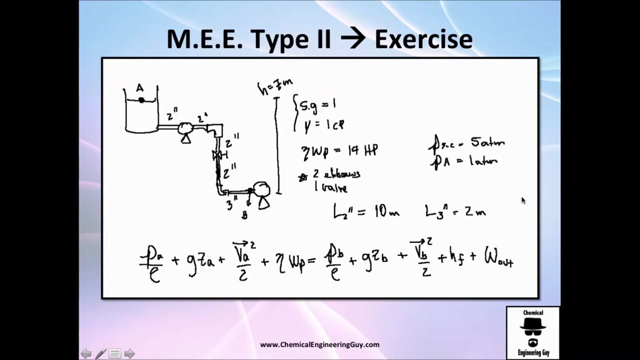 so i'm going to change it to cubic feet per second, because those were the units they were asking us. they were: we have feet, we have inches, so they're asking us to get it in english system. so i round it up and i think three cubic feet per second is my final answer. good, 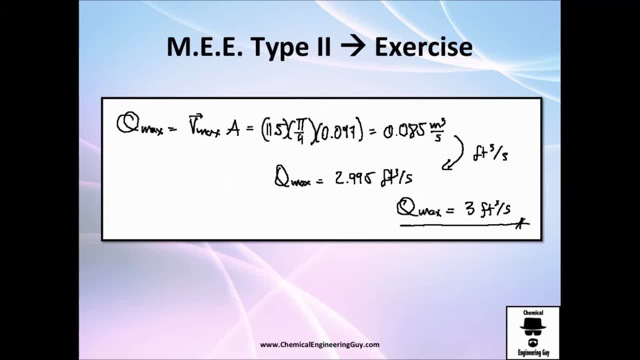 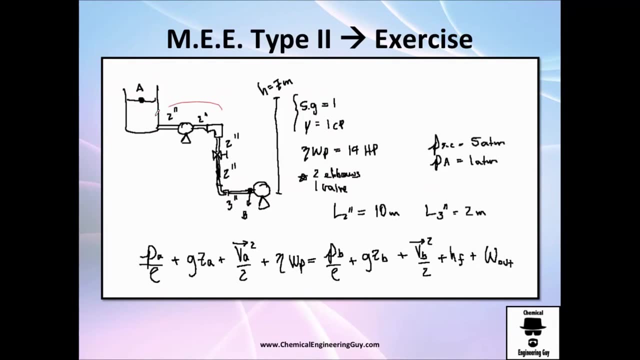 this is another exercise, so i'm going to try it again. so the last exercise was this one: right here, to calculate the volumetric flow rate. we found out we eat three cubic meters per second. but what will happen if we have two pipes, for example, two inch pipe right here and three inch pipe right here? and yeah they, we got. 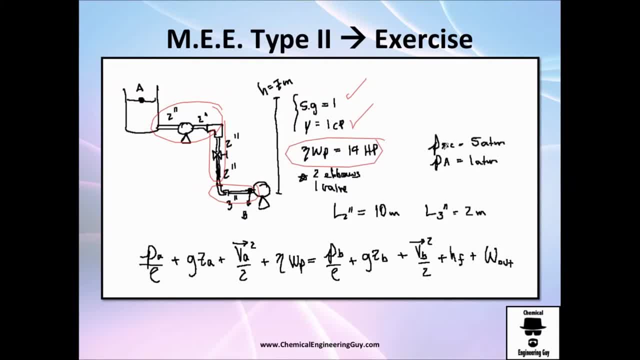 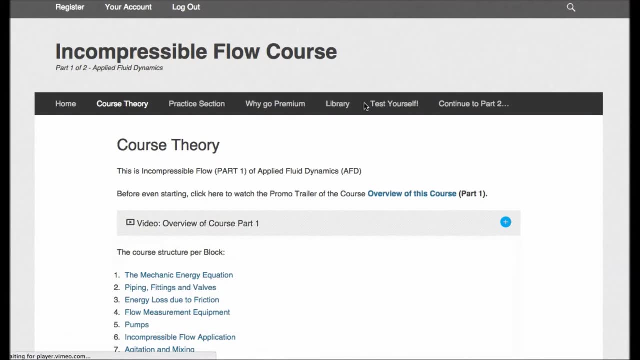 the specific gravity, we got the viscosity, we got the power of the pump, we got found, uh, the suction in the inlet and outlet, got the length of all the pipes and we know all the accessories and also the height of the points. so hey, there, guys, probably you've been watching this course and you've been watching essentially. 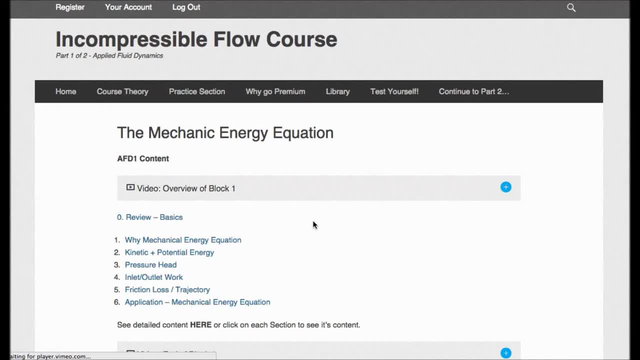 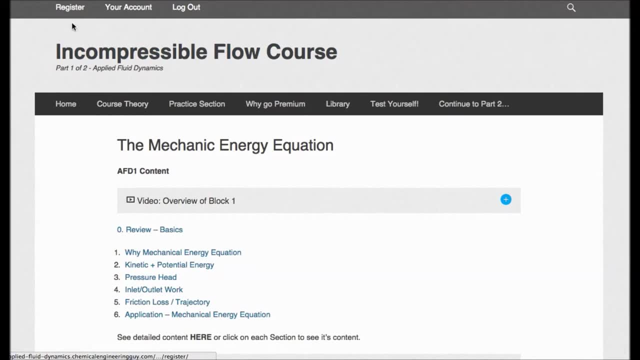 just a section of the course, and not only that. you watch a plenty of ads, if not mine. there are also youtube ads, so if you want to get rid of those, go and register right here. not only that, you will get also high definition content and you will be able to. 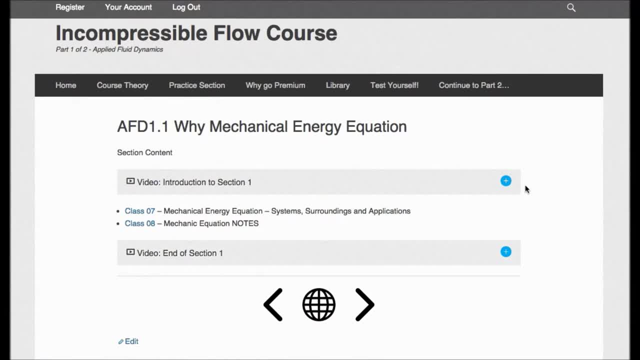 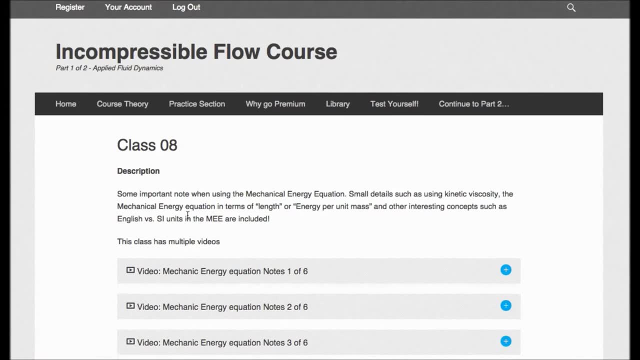 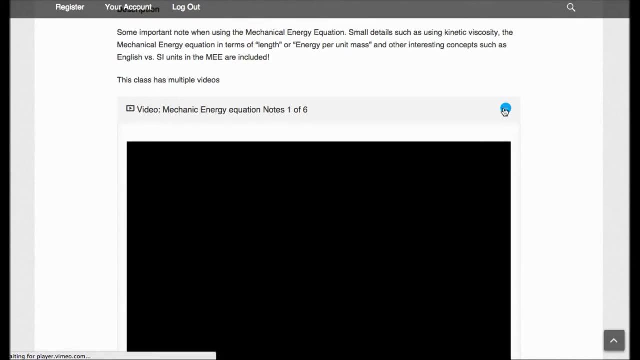 follow the course in a proper way, which is a way more friendly or user-friendly interface and, for instance, if you want to go and check out class 8, you'll be able to read the description, get plenty of videos. so, for example, you get to check out this video and, yeah, essentially you get to see. 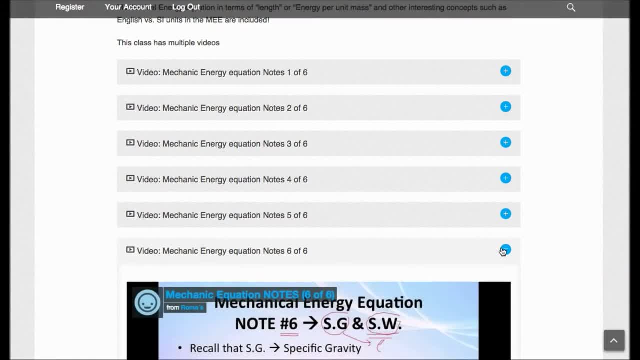 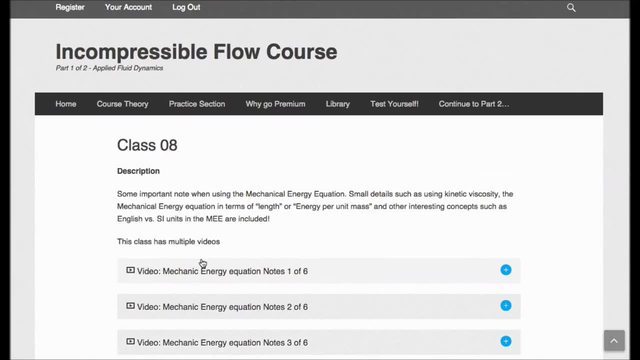 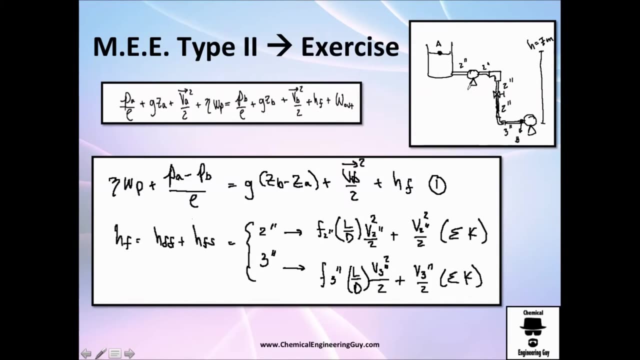 every one of these videos through these tabs. and not only that: if you want to ask any question, you can leave it here in my reply and i will answer you asap. how can we solve this? well, number one, we will need to split this into two problems. 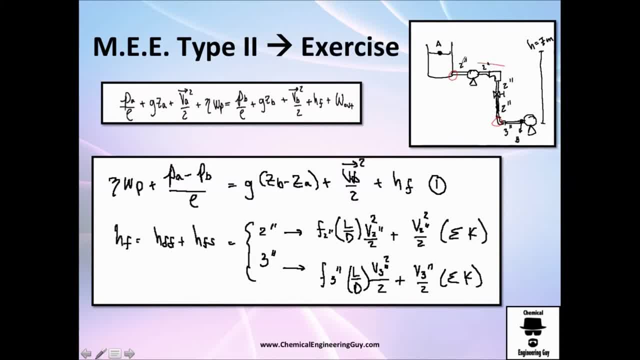 the first problem will be dealing with the friction loss in number two and the other problem will deal with the pipe, which is three inches uh in diameter. so let's do- we do the balance and we have this right here- what we did. we have a little detail: that hf depends on two parameters: the inch, the two inch pipe, and 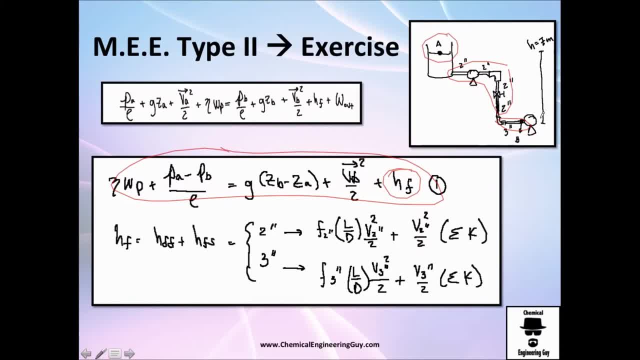 three inch pipe, but the balance is done here, so we have a do, we have it. yes, we have the height velocity zero, so that's why we can sell. so let me actually start doing this. uh, we have. yes, yes, yes, okay, yes, yes, okay, yes, yes, yes, okay. 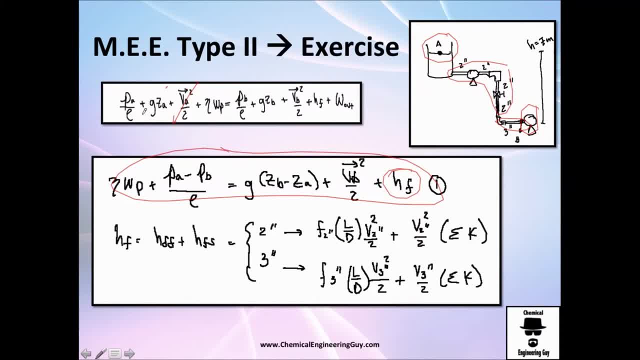 yes, yes, okay. The only thing I can cancel is velocity on A Pressure, and PA and PB are different, so I cannot cancel that. I have a pump, so I cannot cancel that. I got a difference on height, so I cannot cancel that. 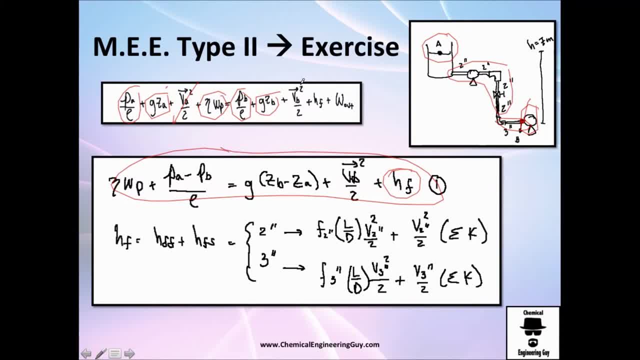 And the velocity analysis is in the suction line so I cannot cancel velocity right here. There is no workout and this is once again the problem. guys, I have this friction factor or loss, or energy loss due to friction, and this depends on pipe number 2 and pipe number 3.. 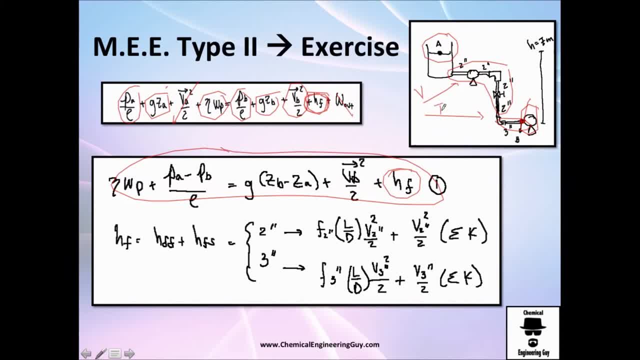 Each one of them has different velocities, different Reynolds numbers, different friction factors and therefore you have different energy loss. So you will need to split this in two: Pipe number 2 and pipe number 3, you do exactly the same as we did before, two times because we have two pipes, and once you calculate the total friction you will be able to solve for the question you are finding, which is probably: what is this pump worth? 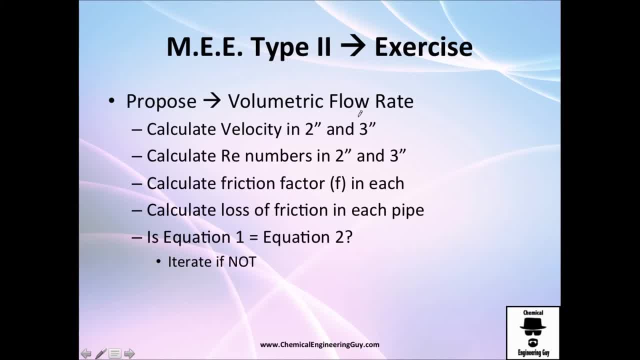 So this is a summary. Proposable dimensions: Volumetric flow rate: always with the volumetric flow rate, calculate velocity in inch or the pipe size 2 inches, pipe size 3 inches. calculate Reynolds number in both pipes. calculate the friction factor in each pipe. calculate the loss of friction in each pipe. 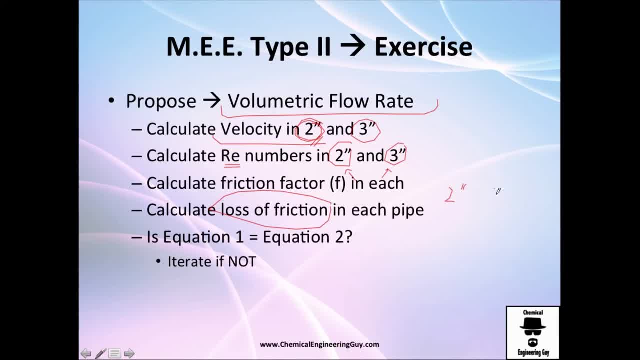 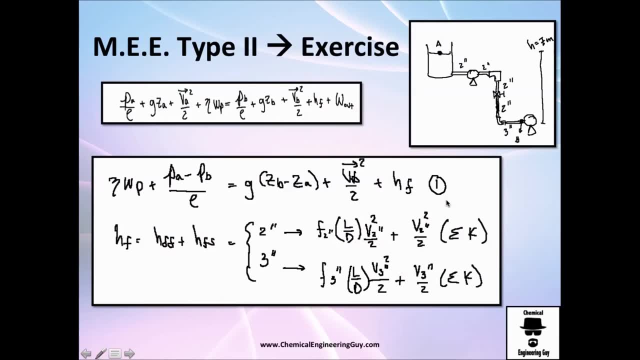 I know it's very tedious, but it's very important to make you understand that we need to calculate the friction loss Separately And now, once we are left, we can finally say if this value right here and this value right here is equal. for example, we got this 3 and we got this maybe 10, then this is not true and you need to propose another volumetric flow rate which will give you another velocity in pipes, in the different pipes, in the 2 inches and in the 3 inches pipe. 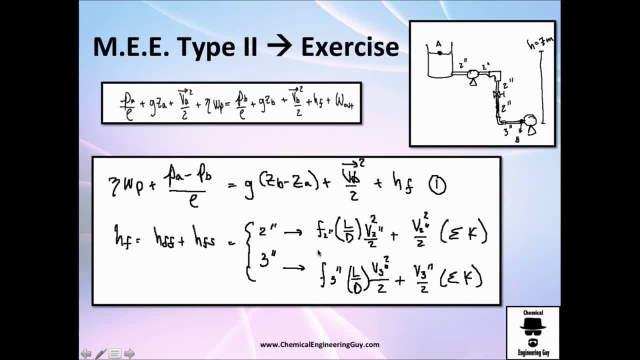 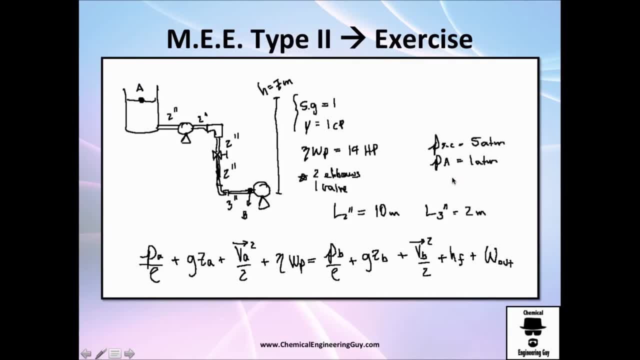 Okay, so just be sure, this was A little bit more complex if you compare it to the first exercise in which we calculated volumetric flow rate, But the idea is the same. Do a balance. Compare this side right here with the right side right here. 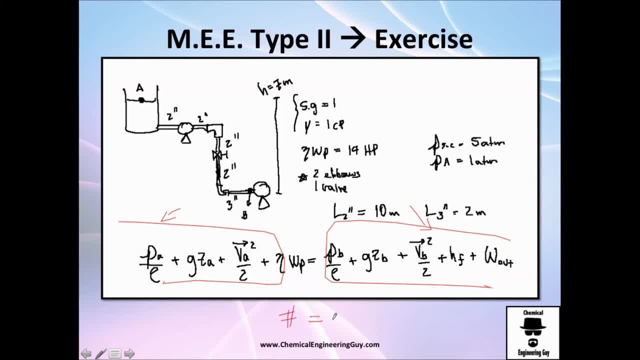 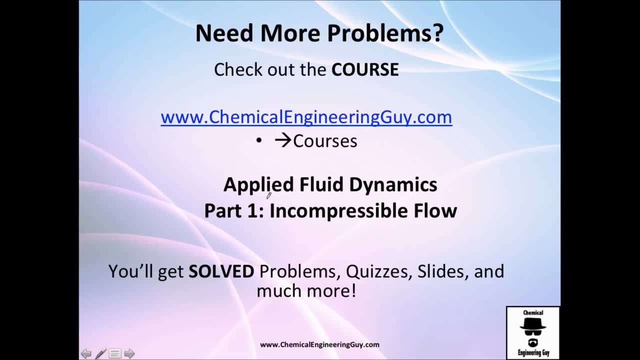 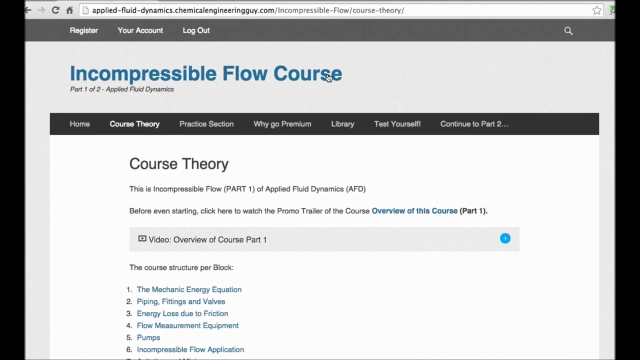 And once you get logical numbers, you are set to dock. So you need more problems, guys. You can find always more at this course right here. part number one: solve the problems, quizzes, slideshow and way much more material. this was a free preview. you want to get full access? go to my incompressible flow course. the link is in the